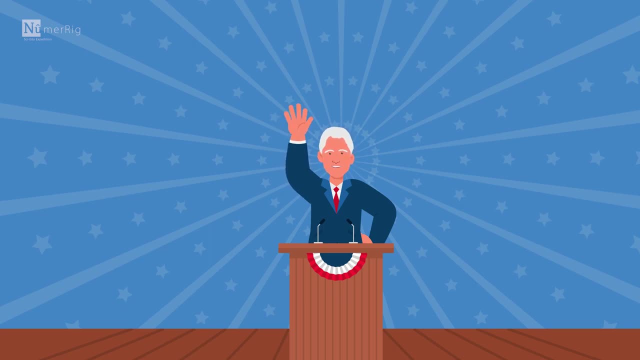 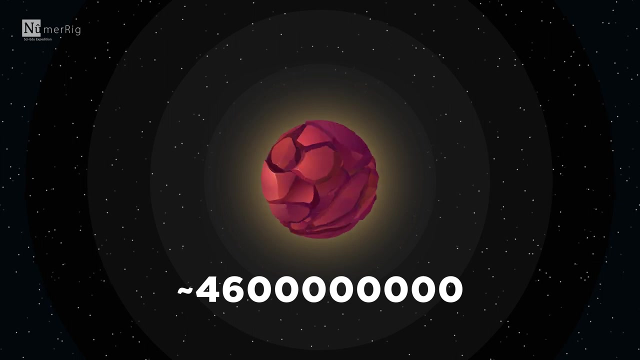 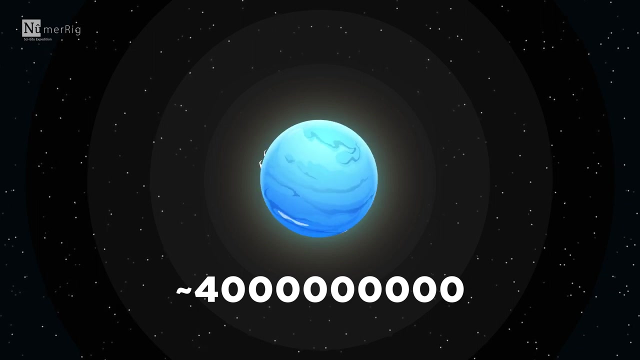 words by Preston Clinton when he unveiled the rock Allen Hills 84001.. The earth was formed 4.6 billion years ago. For millions of years it stayed dormant with no form of life appearing, And then, around 3.7 billion years ago, microorganisms appeared and it became a. 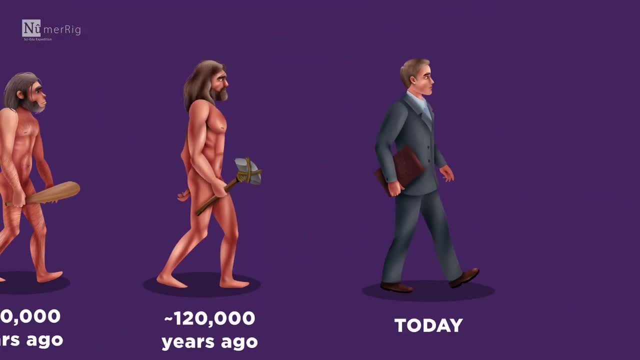 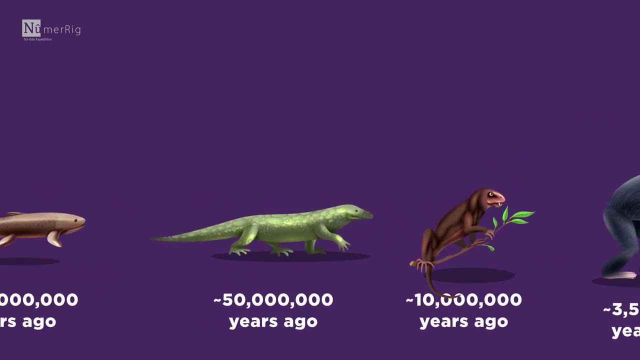 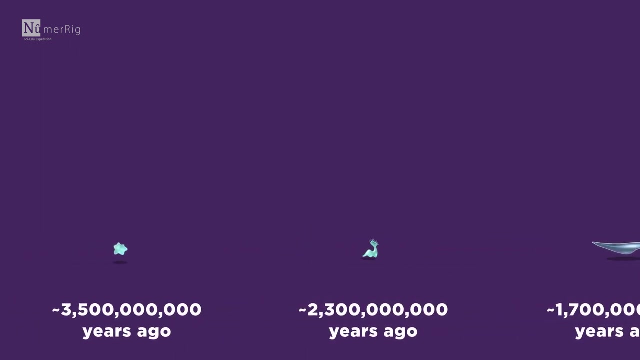 bustling planet full of life. The origin of life on earth remains one of the greatest mysteries of our time. There is no known explanation for what happened 3.7 billion years ago To make the planet home to millions of species. today, a variety of theories and 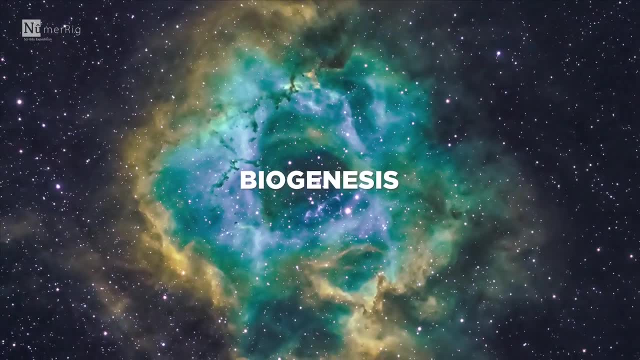 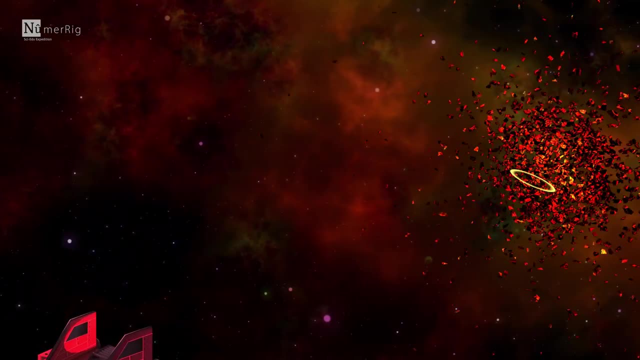 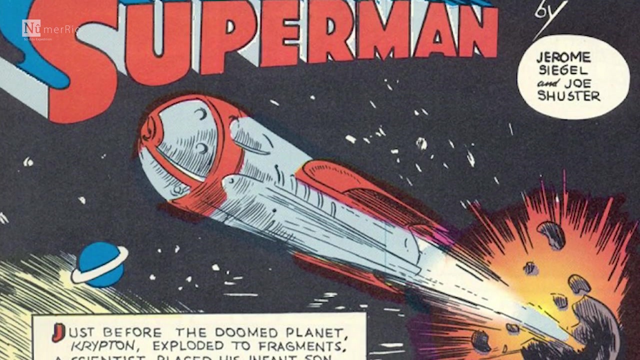 hypotheses have been proposed for explaining and reasoning the origin of life. As the last surviving son of Krypton, Superman, was sent down to earth after his planet was destroyed in DC comics, Maybe we are in so far off from reality as we thought from this comic book history. 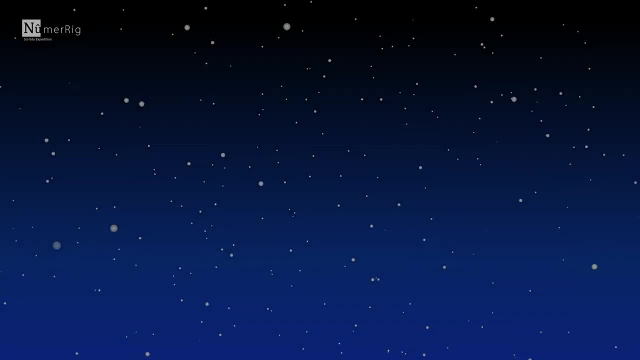 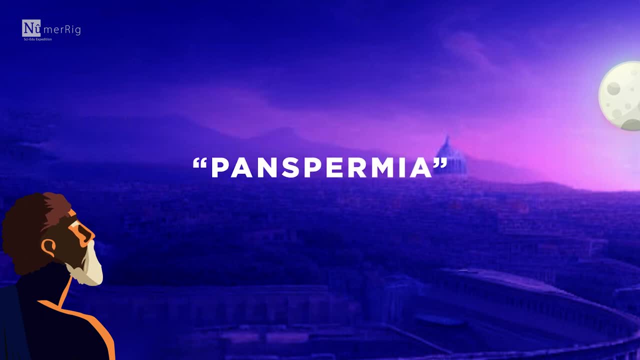 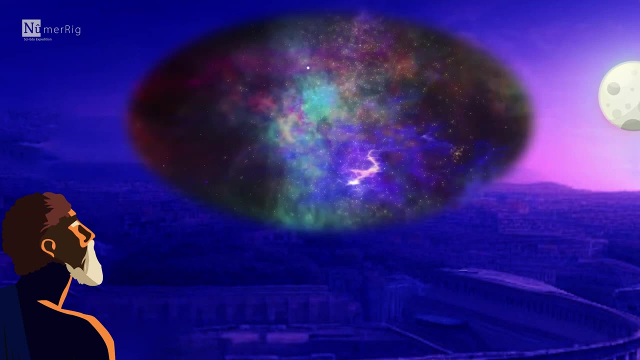 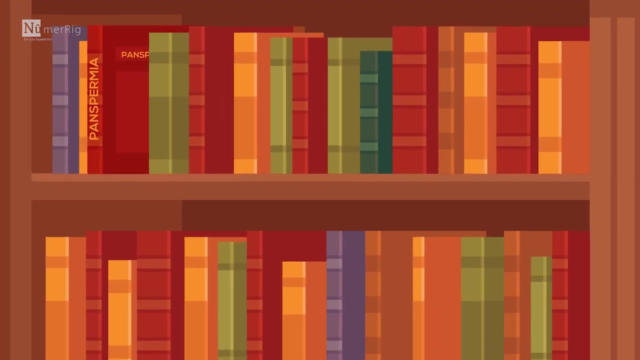 and said Panspermia, which means seeds everywhere. Anaxagoras believed that space is filled with seeds of life soaring across the universe, and not a vacuum. At that time, however, it was not taken seriously and was not mentioned until 1747.. The universe is not a vacuum. The universe is not a. 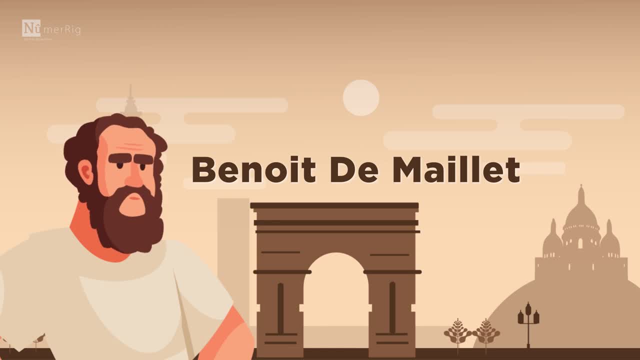 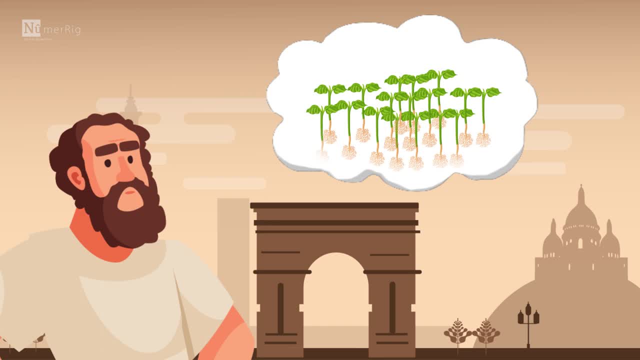 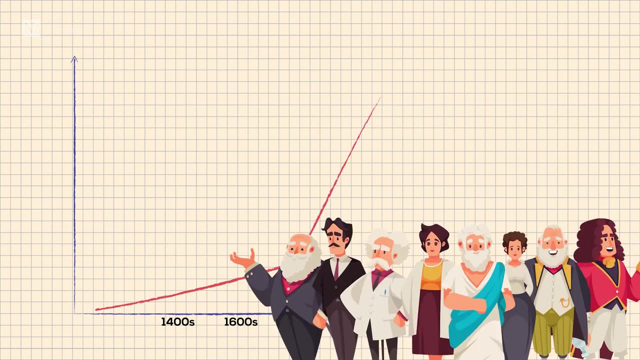 rained down to the oceans from the heavens, and so evolution began. The theory took off in the 1800s, when various scientists suggested that life was planted on earth through stones. When the earth was hit by asteroids and comets, they believed that one of 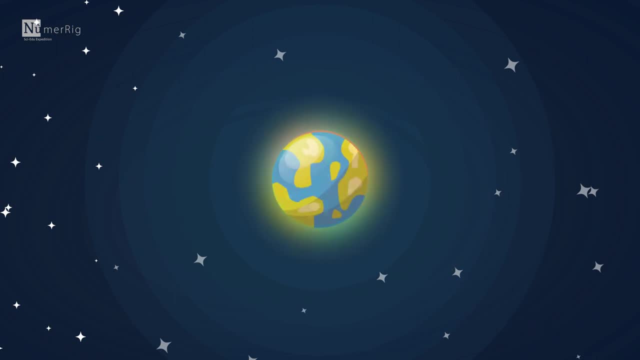 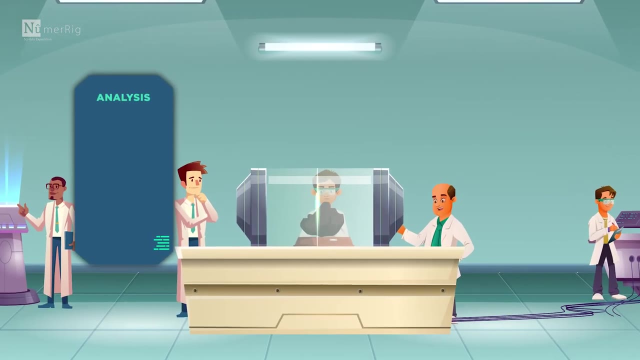 them should have brought the organic molecules necessary to make primitive cells. Meteors falling on earth hit the earth and the earth was hit on the earth through stones. Meteors falling on earth, the earth- are always analyzed for molecules. these days they are often identified with amino acids.